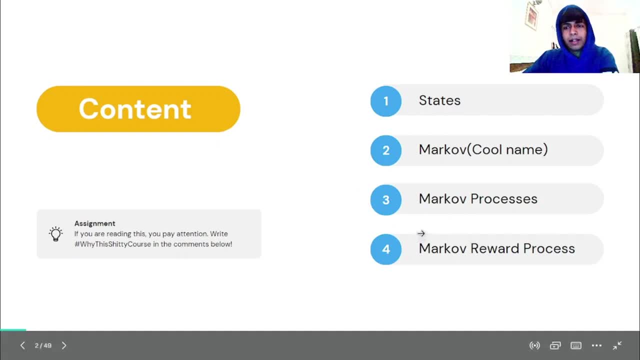 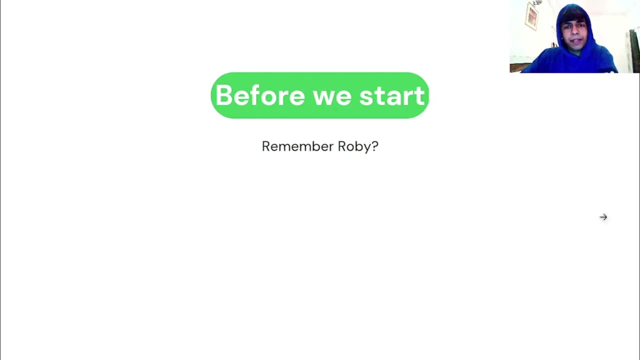 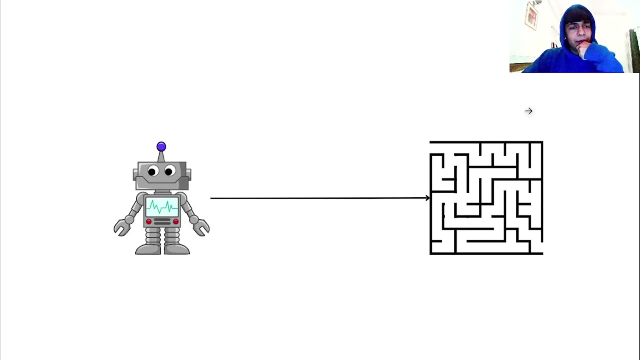 introduction of Markov reward processes in the same video, but we'll discuss it in detail in the next one. So before we start, do you remember Robby? So Robby was this really cute robot who was trying to learn how to walk in this maze. So while doing so, Robby was making intelligent 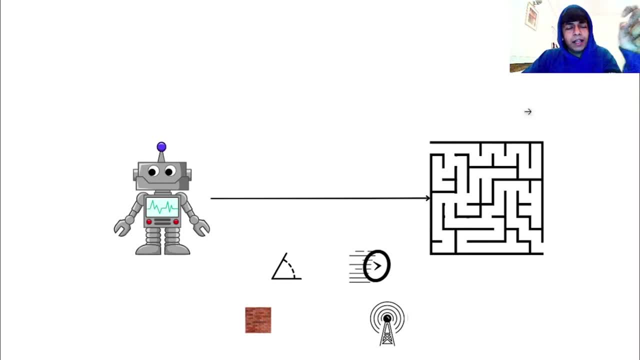 observations such as angle of orientation, the speed where the wall is and the sensory information that was being fed, that was being transmitted by the sensors we have placed on Robby. So all of these together, when grouped, we can term as observations. So does it make sense to you when I say that these observations are enabled by an observable? 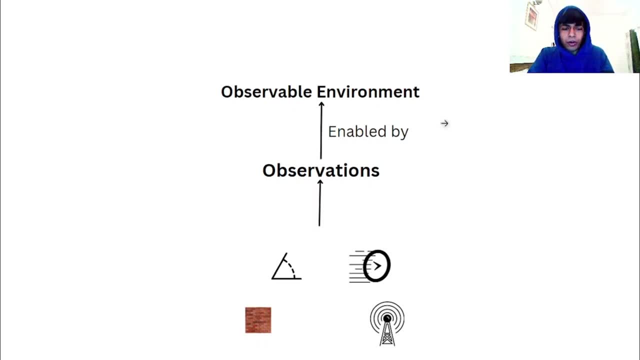 environment. Does it make sense when I say that not only Robby and the sensors and its whole features that Robby comes with in addition to that, these observations are enabled because there is an observable environment. So what do I mean when I say observable environment? 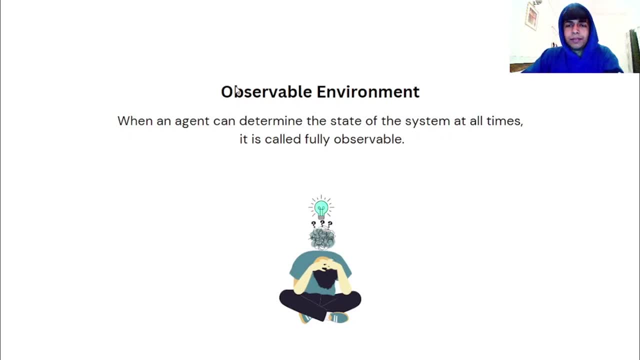 So when an agent can determine the state of the system at all times, it is called fully observable. So it might seem a little daunting at first. but let's just think about a scenario. Let's just imagine you walking down the road and I have given you one task. You don't have to. 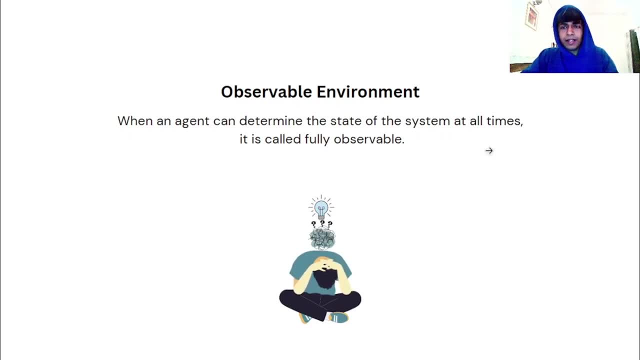 you can't bump into anyone, you can't collide with anyone. and how do you do that? So, in the middle of the day, you have plenty of information, you have all of your five senses and there's plenty of light, so you can see everything clearly. you can see where your fellow pedestrians are. 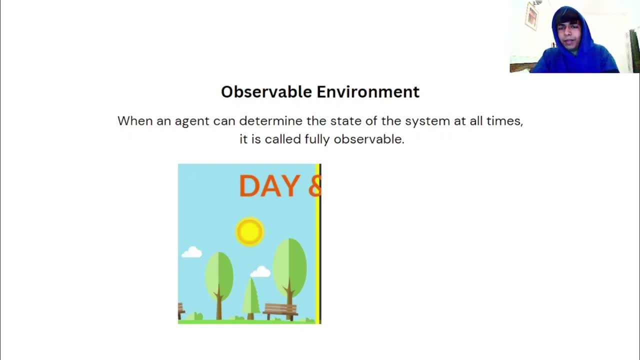 you can see the traffic, so it's very easy to you know, not bump into someone. But if I do the same thing, if I tell you to do the same thing at night, where there is total darkness, so even when you are still able to see, hear, touch, feel, everything like all these five senses are still there, with 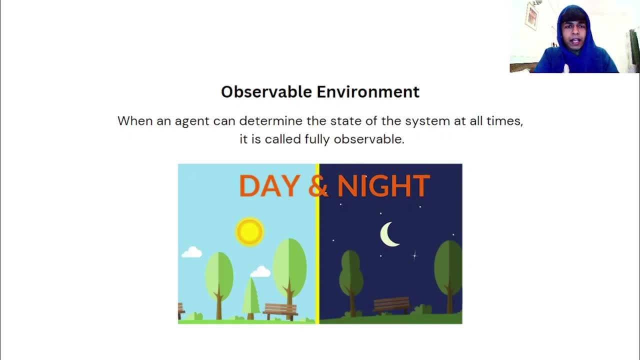 you, but the environment is not enabling you to take in all the information that you actually need. So we can say: during the day the environment is fully observable, whereas during night it is partially observable. Now we'll look forward into what a state is and take a more intuitive example. for the same, 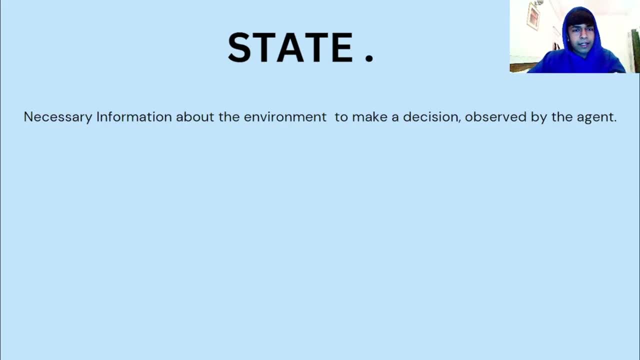 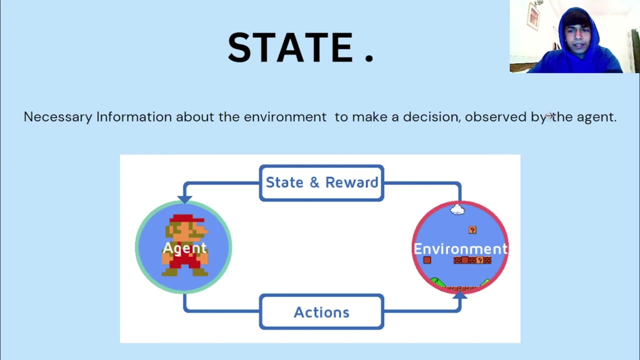 So in the previous video, I defined state as a necessary information about the environment to make a decision observed by the agent. So let's take a very natural example for the same. So Mario, right, every one of us has played Mario. if you have not, I'm really. 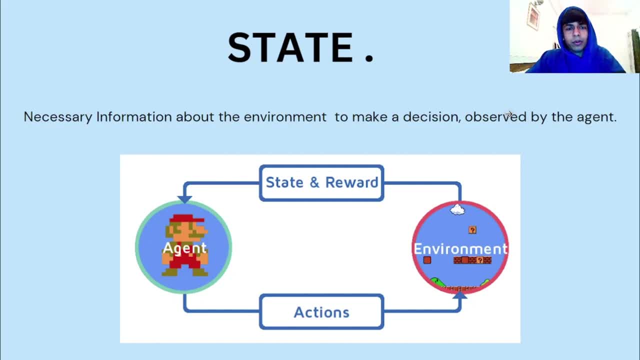 sorry for your childhood, but in Mario, what he's doing is he's trying to level up to ultimately save the princess, right? So the agent or Mario is interacting with the environment to do the same. and what, according to you, will you define as the state of a Mario game? So state can be defined in so many ways. 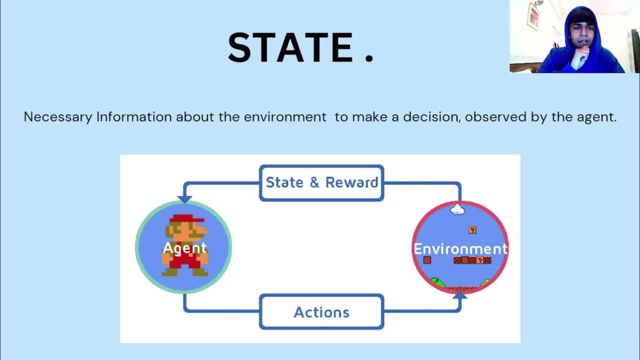 In so many different terms. it can be defined as Mario's position. it can be defined as the level Mario is at. According to me, the information that would entail everything, every necessary information that we would need to help decide Mario what to do next, would be in that screenshot. 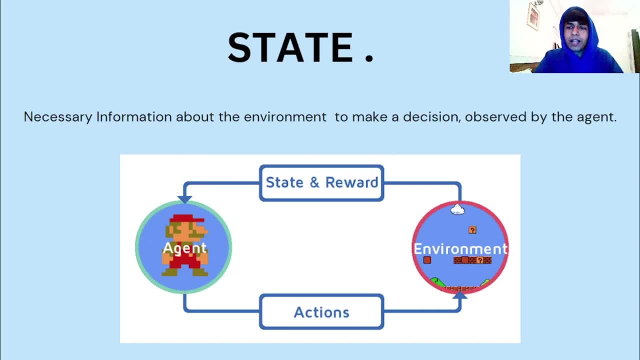 of on that particular time step. The screenshot of the game at that particular time step would be a perfect description of state. It would contain the score. it would contain all the obstacles that Mario has in front of him, or at least the obstacles that we can at least see and hidden. 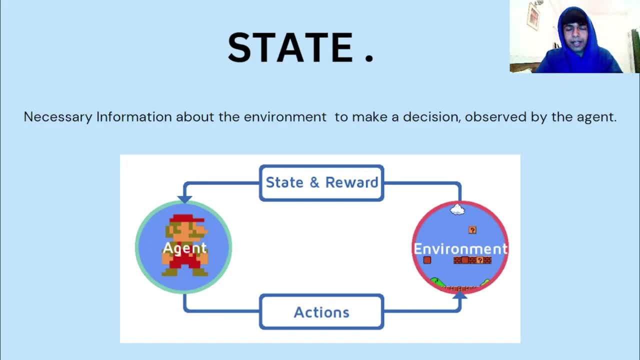 breaks, bonuses, rewards- everything will be encapsulated in that screenshot. So state can have a broad description, but it is best to find that boundary or to find that perfect definition of state. that will help us. that is more relevant to our problem statement. 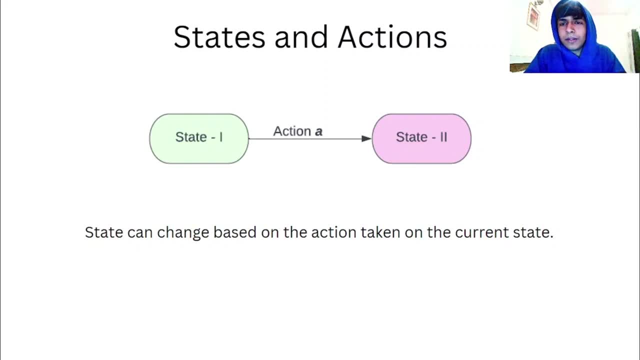 So let's see how states and actions come together. So let's say that we are in an initial state 1 and we undertake an action A. We observe that we move or we transition from a state 1 to state 2.. So we can take a very natural 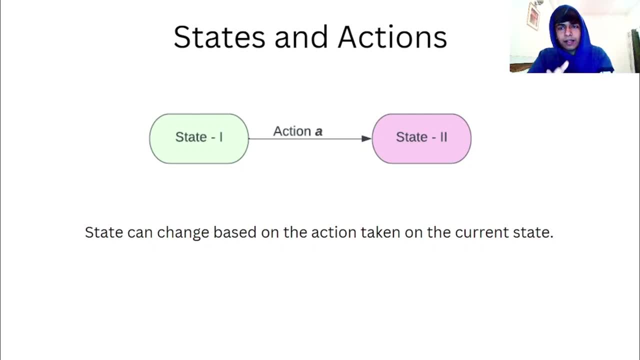 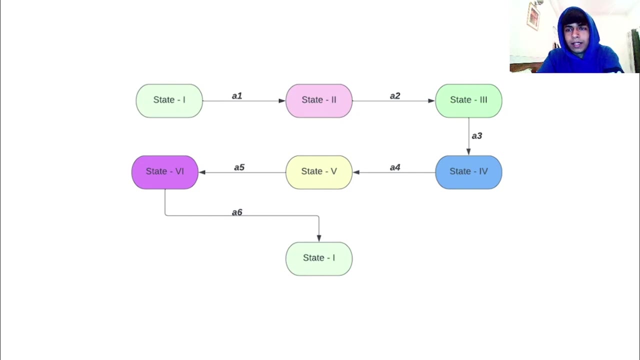 understanding from this that transition in state occurs when we undertake actions. It's a very simple, like, I think, a very intuitive understanding too. So we will see a chain action for the same understanding or the same approach. Let's say that we are in state 1,. 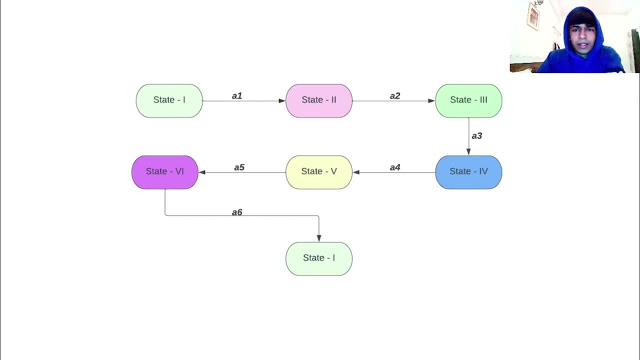 we undertake an action A1,, we go to state 2.. Similarly, state 2 undergoes an action A2, transitions into state 3.. What I want you to do is I want you to draw your attention to this transition itself. State 6 undergoes an action A6 and comes back to state 1.. 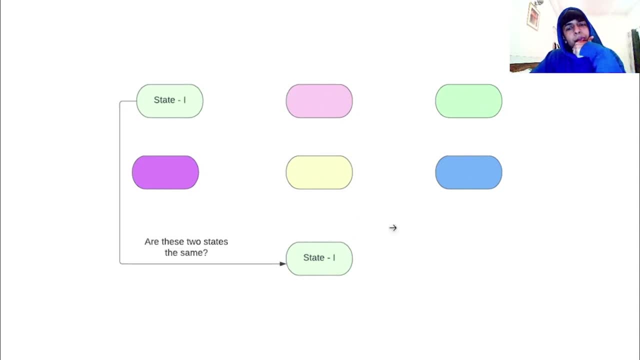 Now I'm going to ask you a very weird question: Are these two states the same? So the way I would have answered this question would be: yes, they are same because they are named the same. but no, it's more than that. What I'm trying to ask you is: in this case, state 1 was an initial 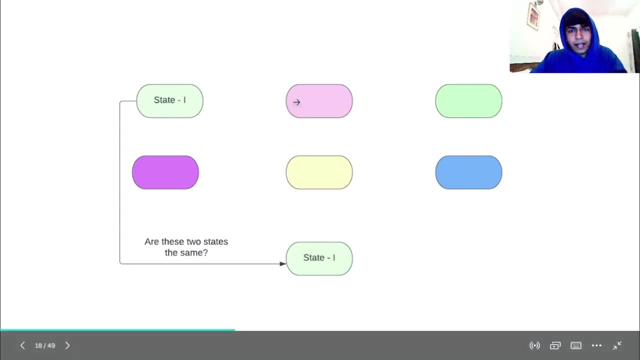 state, In this case state 1, has undergone five intermediary states. So do you think that this state would consider like this state 1, this version of state 1 would have more information as compared to this state, Or are these two states the same? Essentially, if they are Markov states, both of these states are the same. 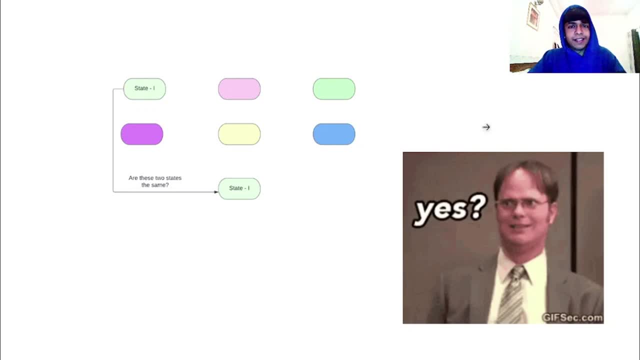 And it's very interesting to actually build an understanding of this. Let's take another example: before even defining Markov, Let's take another example, in C, and build an intuition or build in like understanding of the concept of Markov properties. Let's say we are interested. 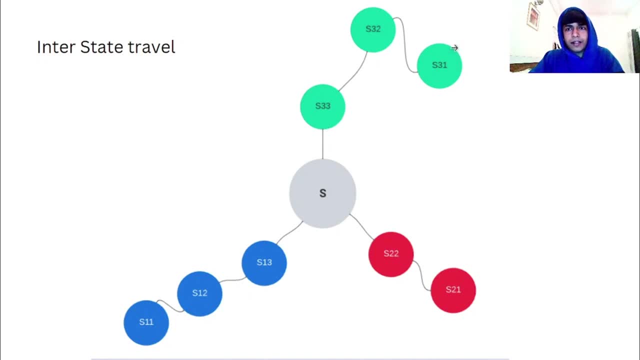 in this state S, and we can reach this state S through three different roads: A red road, a green road, I guess, and a blue road. So all of these three roads are mutually independent. They have no connection to each other. So what I want to ask you is that the information that 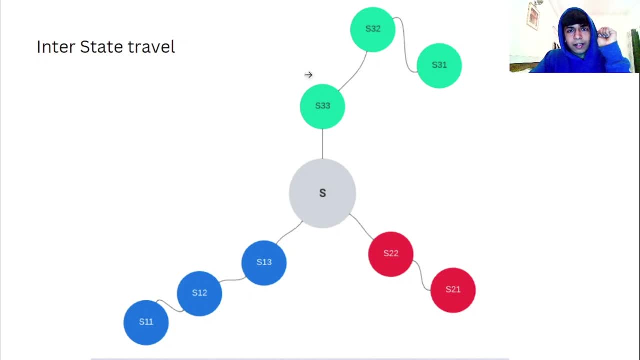 is stored in state S when we enter it through the green road. is it different than the information that state S would contain when we enter it through the red road? The answer is no. The information that the state S would entail or would contain within itself will be independent. 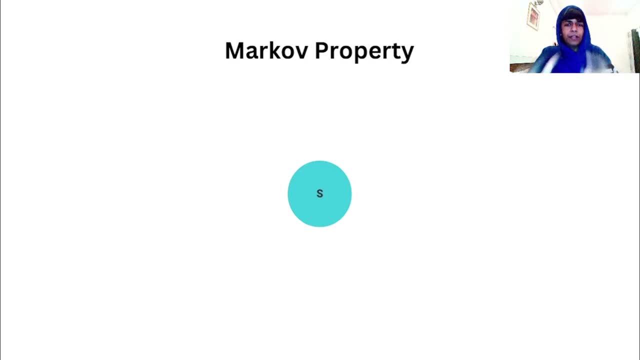 of what states it has gone through to reach state S. So a very famous Instagram quote I think almost all of you would have heard is: the future is dependent only on what you do in the present, not in the past. So this is what Markov property tries to say. It says that the state, the present, 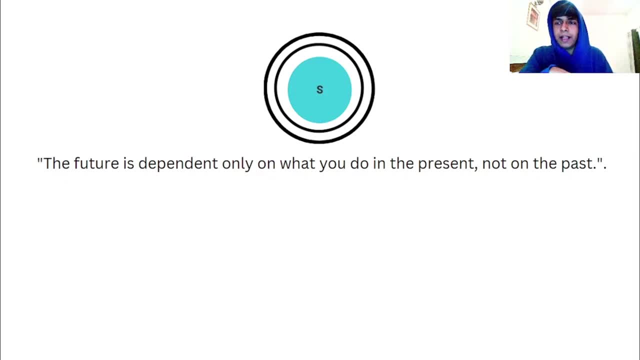 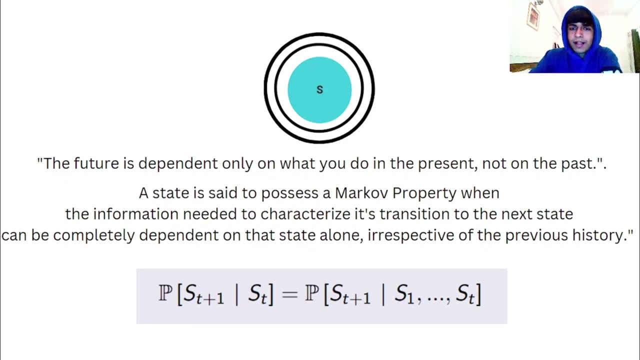 that is necessary to characterize what you want to do or what decision you have to make. All that information that you would need is in that present state itself, and you do not have to worry about the history or how we got to that current state. So this is the same expression. 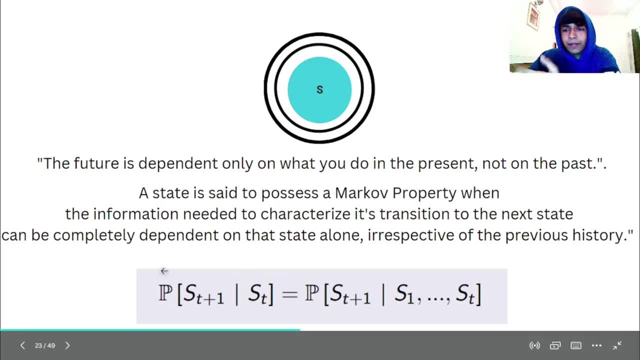 with just a formal definition. I will not read that out loud. Even I don't understand it, So let's focus on this expression here. The expression states that the probability of the future state or the state at t plus one, conditioned on the information that the present 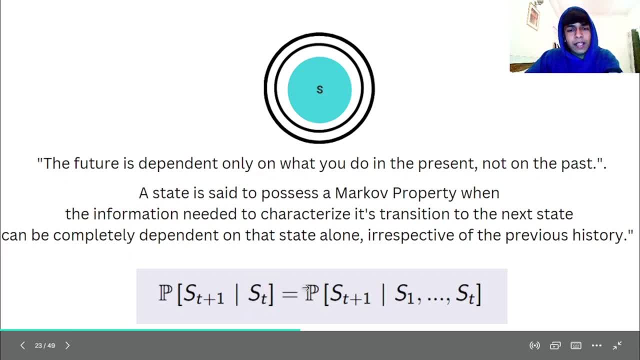 state is S of t is equal to the probability of the future state, conditioned on the information of all the states that have been visited until time. step t, which means that the information that the whole history of states is giving us is equal to the information of the current state. 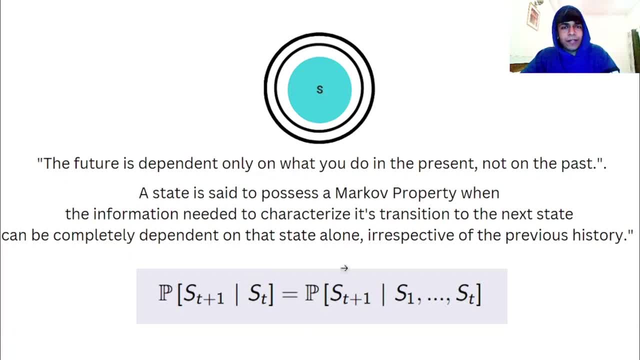 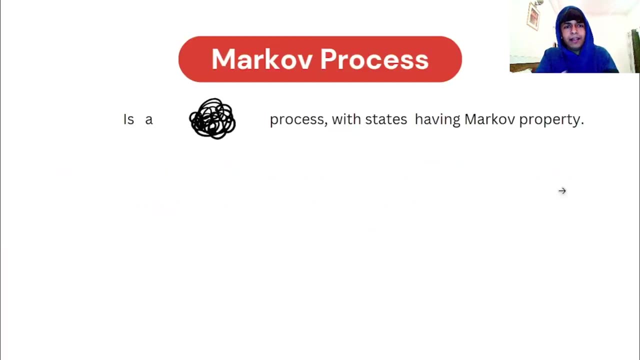 itself. So we do not even have to worry about the history, We just have to worry about the present. It is good to go on any information that you would need to take any decisions on the future states, Right? So that's what I mean by Markov property. So what is a Markov process? 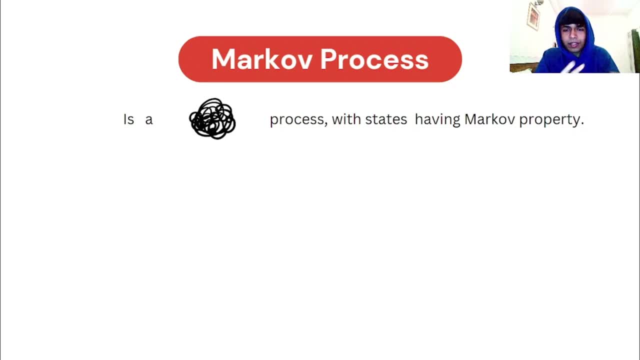 So Markov process, to be correctly categorized, would be a random process. It is a random process with states having Markov property. So Markov process is a process with Markov states. It's as simple as that. So let's take a very simple example. So we have four states here: S1, S2, S3, S4.. 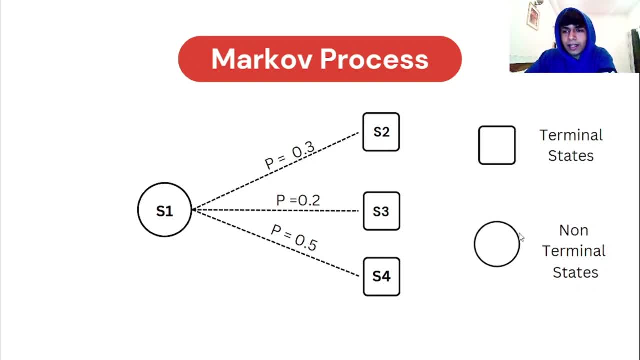 So I have denoted terminal states by squares and circular states by non-terminal states. So terminal states, what do I mean by them? Terminal states is self-explanatory, that the process ends there. If any transition of any state leads it to a terminal state, the process ends So in this state. 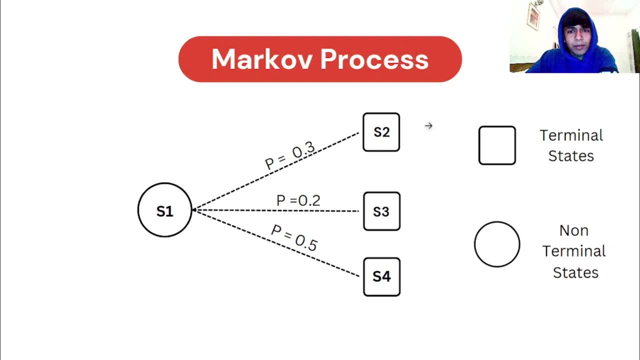 we can see that the state S1 has probability for each transition. So the probability of transitioning from state S1 to S2 is 0.3, transitioning from state S1 to S3 is 0.2 and S1 to S4 is 0.5.. You sum: 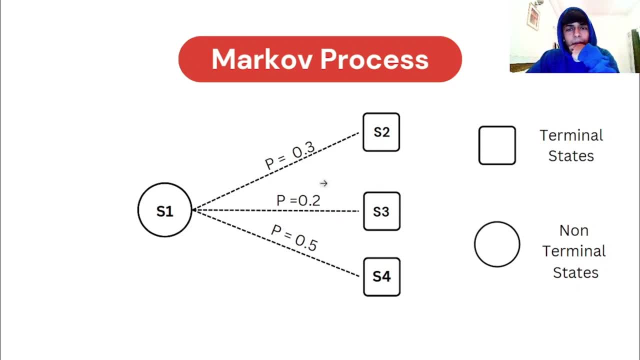 them up, you will come. you will realize that the probability is coming to be one and that is because we know all the possible states. S1 can go into right. So let's take a little bit more complicated example of a Markov process and consider it. Markov state is a state where S1 is 0.2 and S1 is 0.3. So 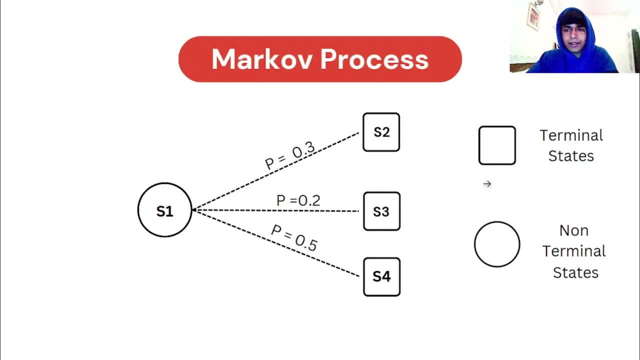 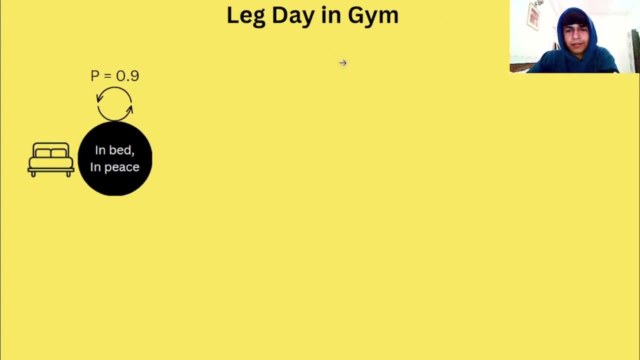 and transition and state transitions with probabilities. right, let's say that you have a leg day in gym, all right. this is, i think, mostly like fitness enthusiast would relate to. but yeah, you, let's say that the initial state is that you are in bed, you are in peace and there is a 0.9. 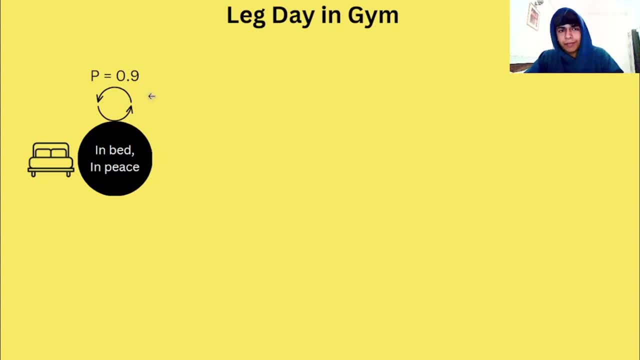 probability that at each time, that at each time step, you would choose to stay in bed and in peace, and you know what? i don't blame you. so let's say that, on the chance that you do decide to get up and you make it to the gym entrance, you're still not in the gym yet. all right, there is still a 0.1. 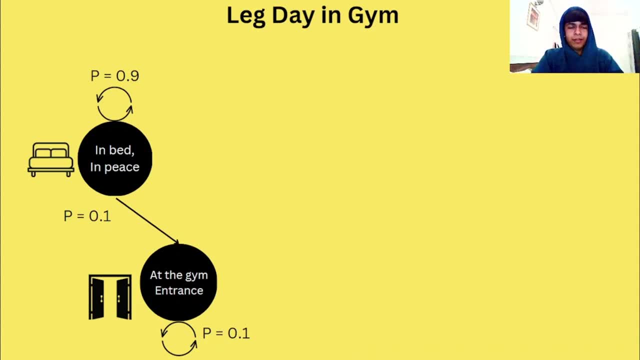 percent chance that you will stay at the gym entrance because you're indecisive of what to do next. then you come up with the idea that you have two options. first is you can go and train legs or you can have sunday on a leg day. so the probability 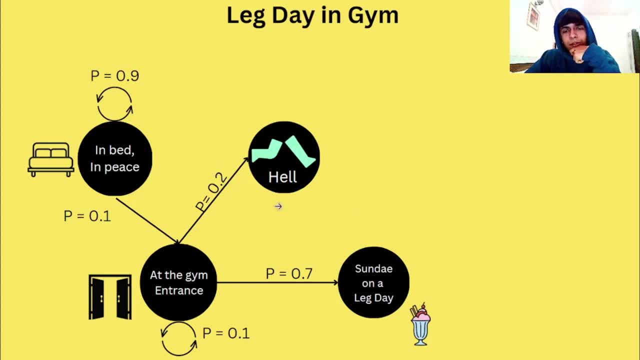 of doing leg day is 0.2 and to have a sunday is 0.7. so odds lie heavily in the favor of having a sunday. but don't worry, even after you go to gym you will still be able to- you know- have a sunday. 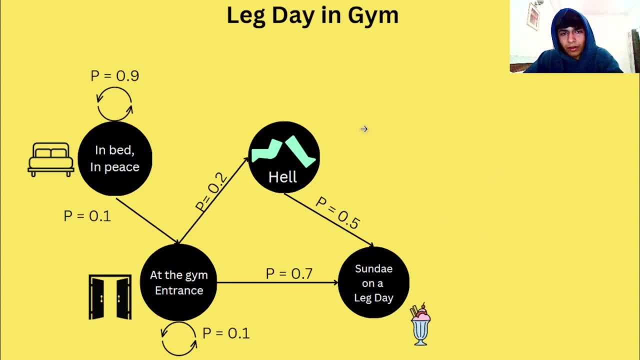 that won't be a problem, and after all of this you deserve rest. all right, so with a probability of 0.5, from the gym you will go to sleep and from sunday you're surely like, with probability equal to 1, you're going to go and crash. so this is a very simple example. 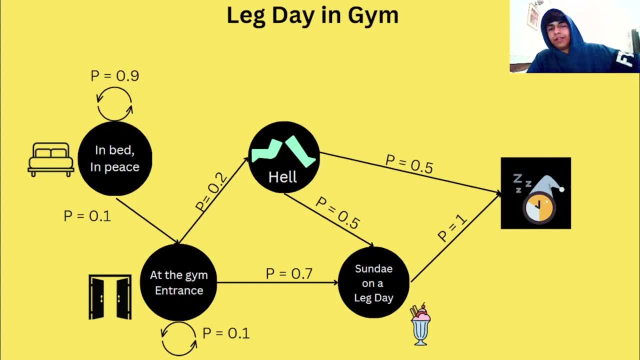 or let's say, a little bit more of a complicated example than we saw in the last, of a markup process. i want you to understand. i want you to just take a step back, pause this and see that. what is a markup process? what does a markup process comprise of? it comprises of states. 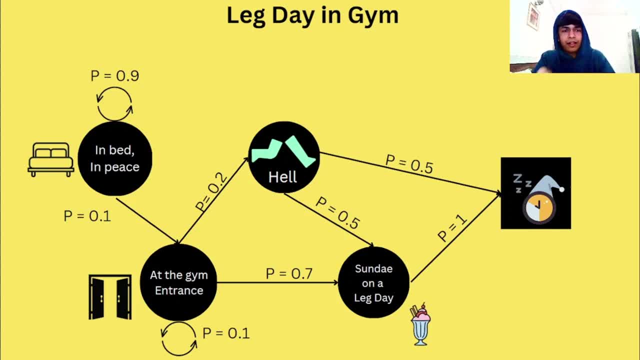 and probabilities, and each state transition has a probability associated with it and i think it's very intuitive to also understand that each transition for each state would always add up to one right, like for in bed in peace. this state has two transitions: 0.9- 0.1 adds up to one right a leg. when you are in the gym, you have two. 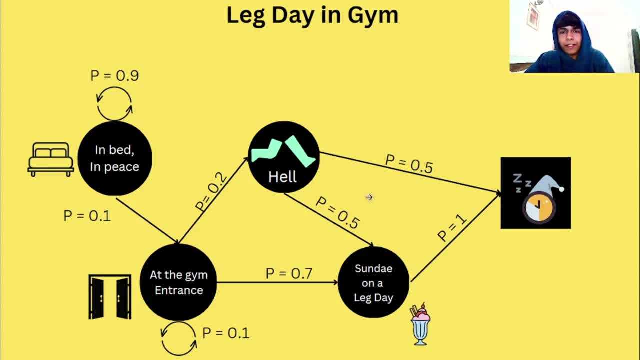 probabilities. you can either go to sleep, you can either go to have a sunday. 0.5- 0.5 adds up to one. so i want you to notice these little things because i think it will help you in the future in the next part of the video. so there is a side quest i'm giving you. what you have to do is you. 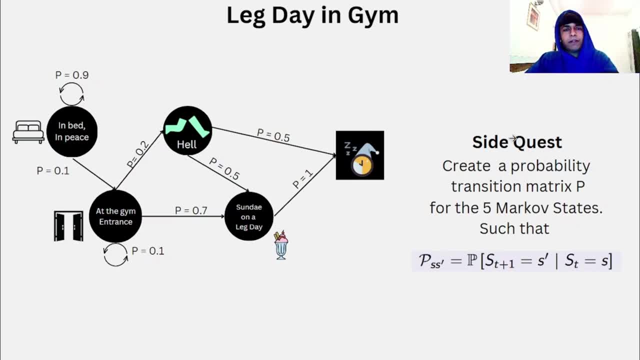 have to create a probability transition matrix p for the five markup states. all right, so what you can do is you can, uh, like a matrix is like rows and columns, right, so you can make one. uh, you can, on the on this side. on the vertical side, you can list all the states and on the horizontal side, you. 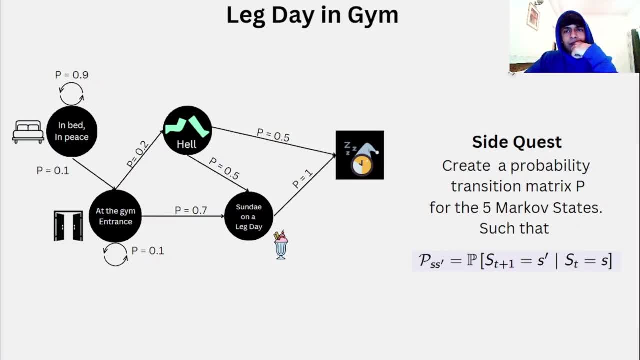 can also list all the states and you can just uh create a probability transition matrix for each state. for m, comma n, like for this expression will make it more clear. so for p ss dash of that transition matrix it will denote the probability that a time plus that the state at 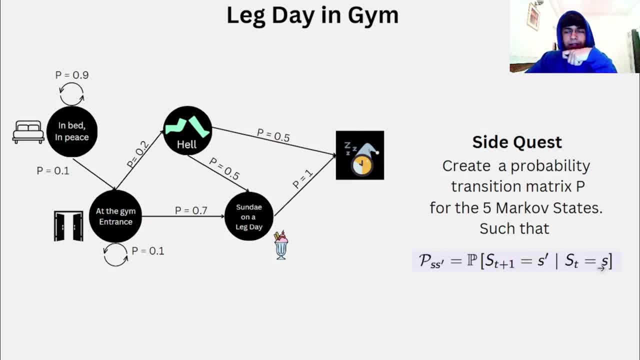 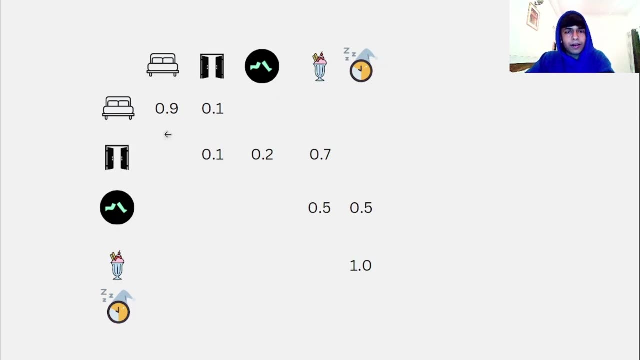 t plus one is as dash, given that the present state is s all right. so pause your, pause the video, make the probability transition matrix and try to match it with the next frame. yeah, so your transition matrix should look like this now if you look closely. the fact that i said that each state 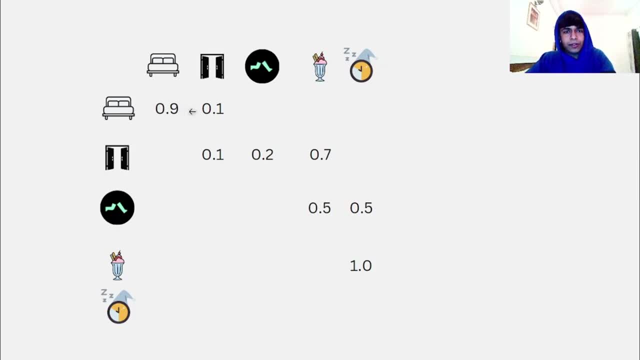 would have each state's probability, transitions would sum up to one. so you can see that each row here sums up to one. so we do not worry about the uh probability of transition states in terminal states. so because, of course, where do you go from a terminal state, right? so we do not worry. 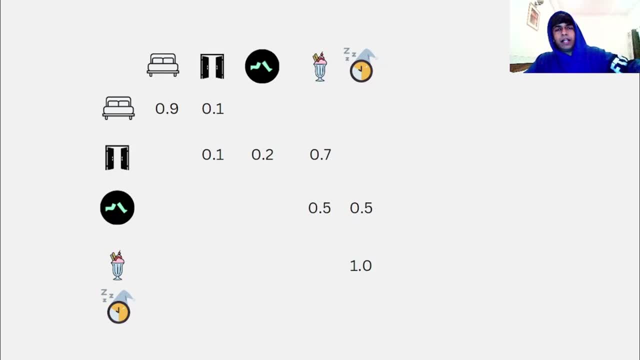 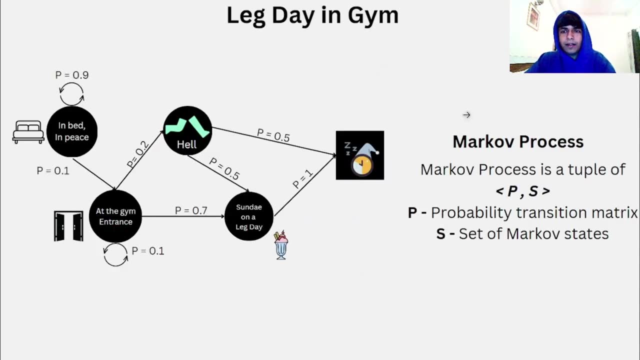 about that. uh, and that is what i want you to take away from probability transition matrix in a markov process, right? so let's just summarize what a markov process, is right? uh, we can easily define markov process as a tuple of p and s, whereas p is the 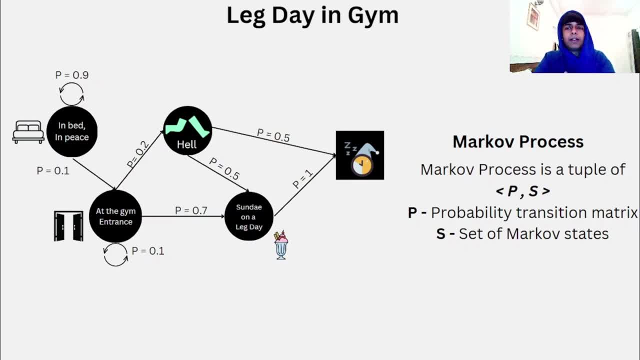 probability transition matrix and s is the set of all markov states, right? so next up, i think we'll be uh looking at markov reward processes and just a little bit intro to them. uh, to make sure for the next video you're geared up for all the information you. 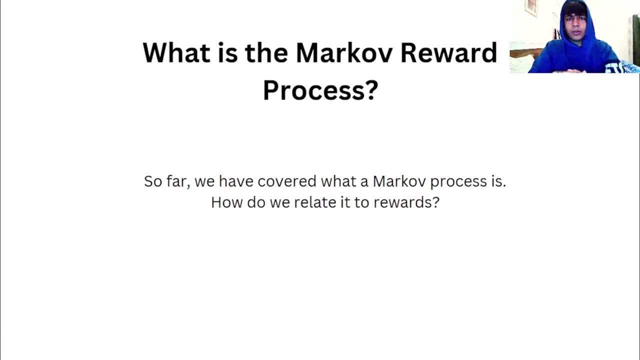 would need to understand the concepts. so what is the mark of reward process? uh, so far, uh, we have covered what a markov process is right. and what do you use to characterize a markup process? you use a tuple of two variables, which are p and s, s being the set of all markov. 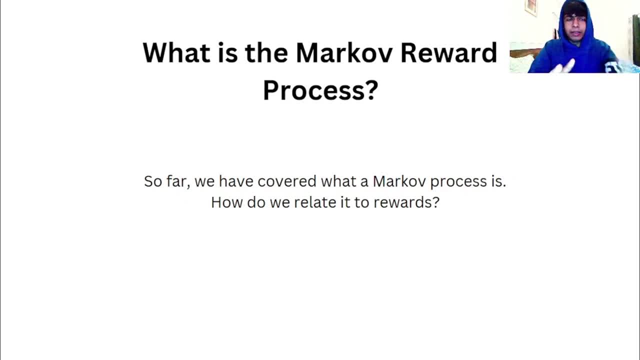 states comprising the process, p being the probability transition state matrix, right being transitioning from a mark of process to a mark of reward process by introducing two new variables to the double, the two of them being r and gamma. so r is the reward which is associated with a particular state and gamma is the discount factor. so what do i mean when i say that reward r? 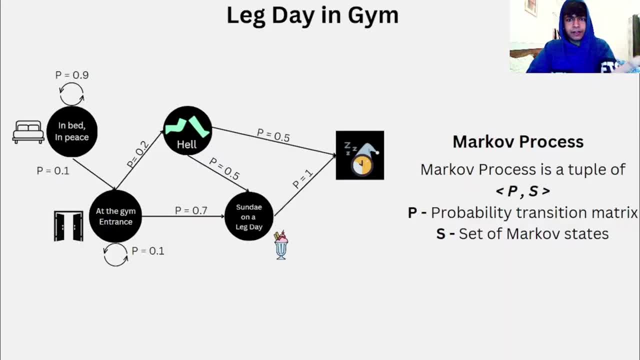 is associated with a particular state. let's just go back a few slides right. let's say that being in bed and in peace has a negative reward and being at the general of the state of counterpoint order assigned in bed respectivist a negative reward and being at the general of the state. right hand side component. 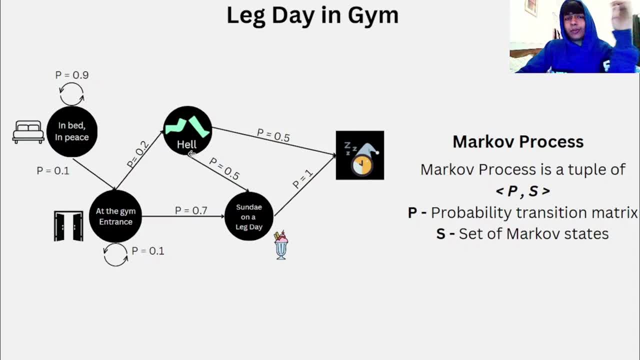 So we have a row on which it says that if we make a decision we have to. calculating the number of objects at the gym. entrance has zero reward, and actually going through with it and training your legs at leg day in gym has the highest reward of all of these five markup states. so this is what i mean. 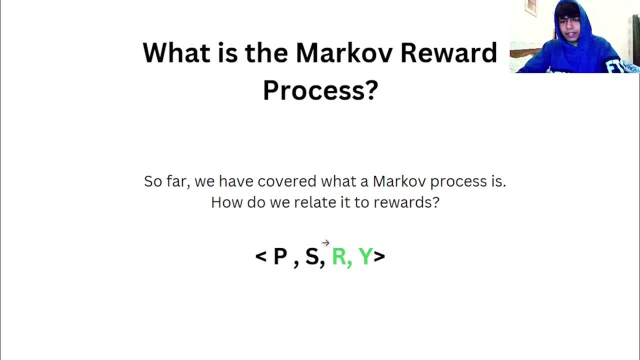 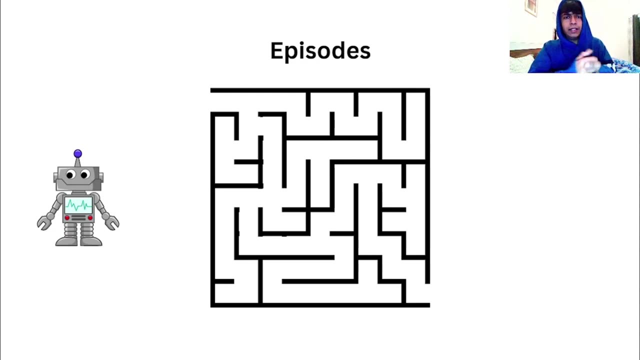 when i say that a reward is associated with a particular state, all right. and to understand what gamma or the discount factor means, we will understand two very simple concepts: episodes, and so let's just start with episodes. so, to take a very simple example, all Netflix series are broken. 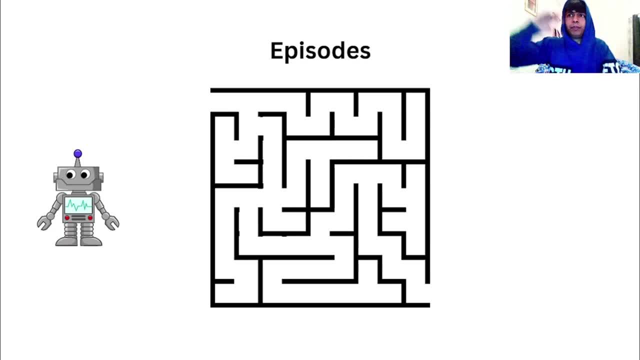 down into episodes, and each episode contributes to the bigger picture or to the bigger goal of the story, right? so the bigger goal is divided into smaller ones and each of them is characterized into an episode. so same is the case with episodes and reinforcement learning. let's just say let's. 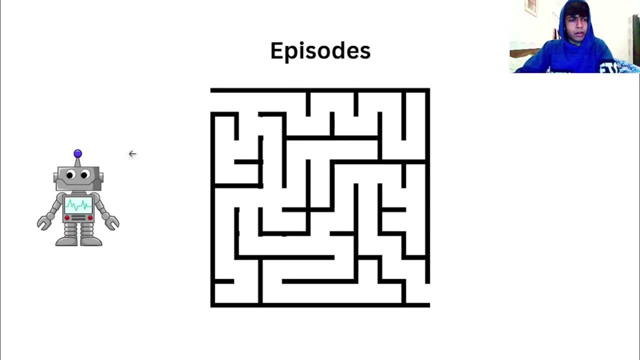 take an example of what an episode for Robbie would look like. let's just first label the entry and exits of the maze. all right, and the initial state of Robbie would be when he enters the maze and the terminal state would be when he exits it. all right, let's 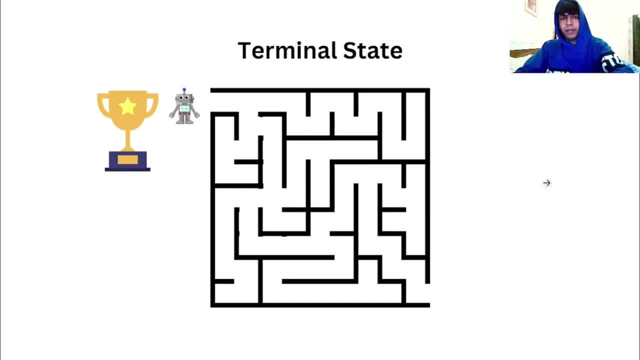 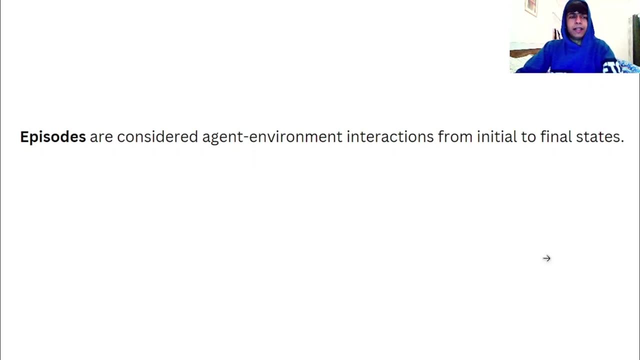 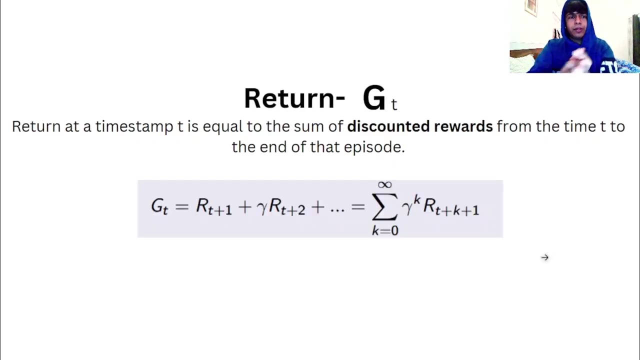 just say that the between the initial and the terminal state between Robbie navigating the maze once in its entirety would be one episode. all right, so episodes can be considered to be agent environment interactions from initial to final states. now we'll move on to understand return. so return at a timestamp T is equal to the sum of discounted. 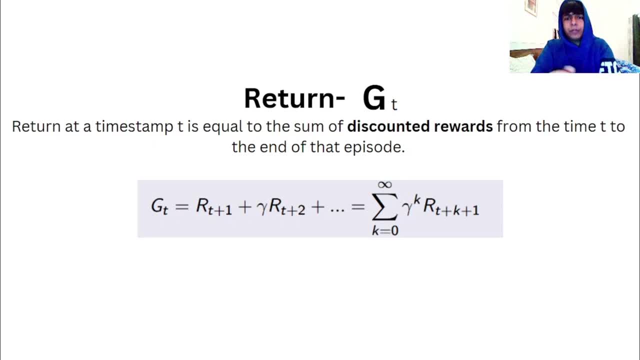 rewards from timestamp T onwards to the end of that episode. so let's just say that. so this expression here you can actually observe that as the timestamp would increase, the power of gamma or the discount factor here would increase. so let's look at the previous example, right? so let's take. let's look a little bit closer into what 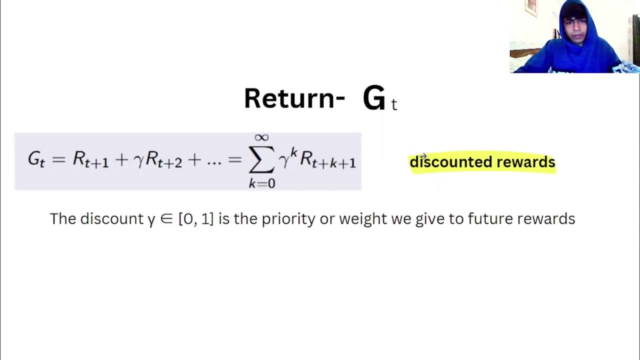 discount factor actually means all right. so discounted rewards are actually discounted by this factor, which lies between 0 and 1 and is actually a quantitative representation of the priority or the weight we are giving to future rewards. so you can have a bit of an intuition by looking at this. 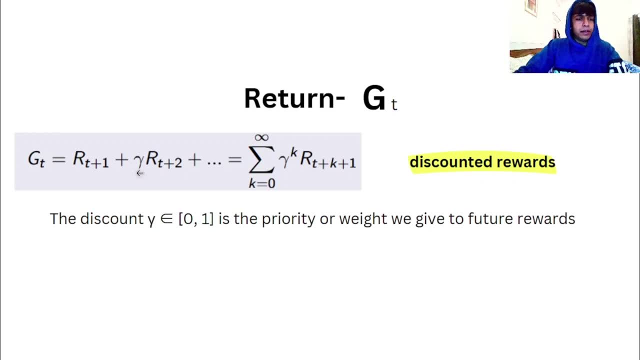 expression here. what if I put the discount or the discount factor and zero, then the only weight or the only priority will be given to the next immediate reward. so it will be a very impatient, or let's just say a very impatient- return function, and a very patient return function would give. 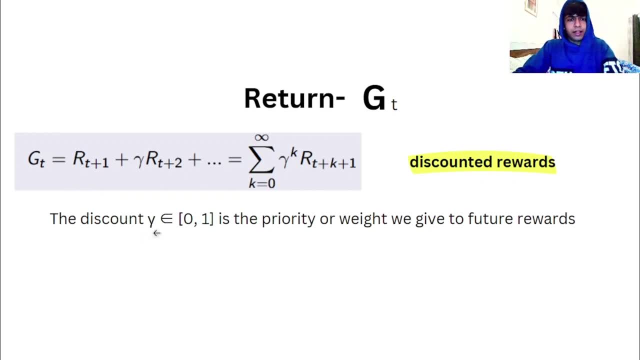 weights to future rewards as well. all right, let's say, if my gava is 0.9, then I am thinking far ahead. I am giving weights to future rewards as well. but why even keep it 0.9? why just keep it? why just not keep it at want? why? 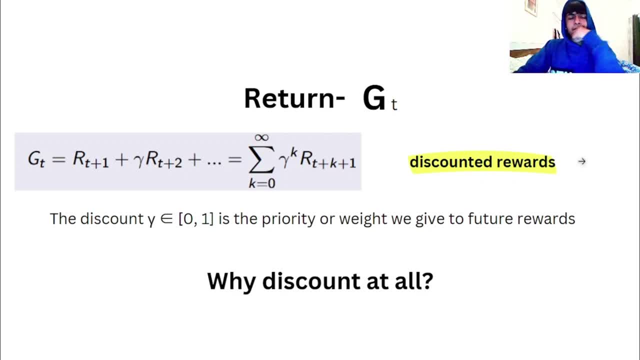 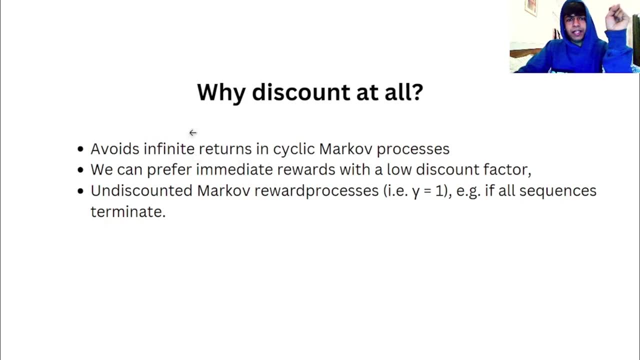 discount at all. so let's just imagine what will happen if you don't discount. if we don't discount, we might get infinite returns in a cyclic mark-off process. so let's just say we understand, we have taken look at. mark of process is what mark-off work process. 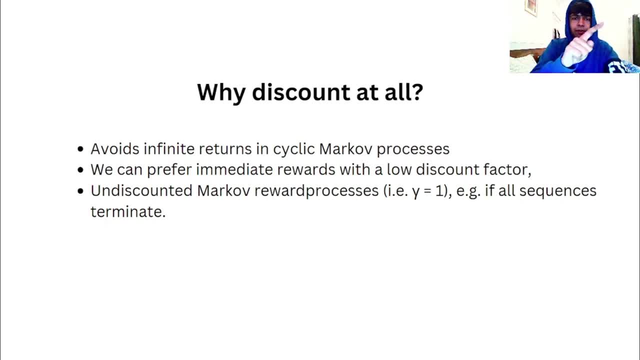 of processes look like. let's just imagine what would happen if a markup process is cyclic, which means that the return would always, always increase, and if we don't do anything to scale it, then we will get infinite returns which we can't scale right, which is not suitable for comparing or even